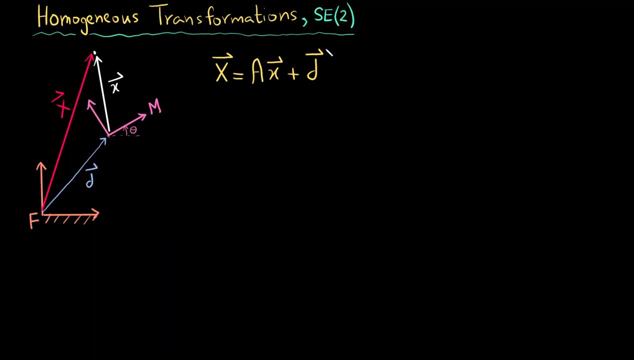 equation right here which helps us to move from the small x to the big X. If I write it out more explicitly, with the big X and Y as the small x vector being a point, x and y and the d vector being dx and dy, and if i replace these terms in the equation here: 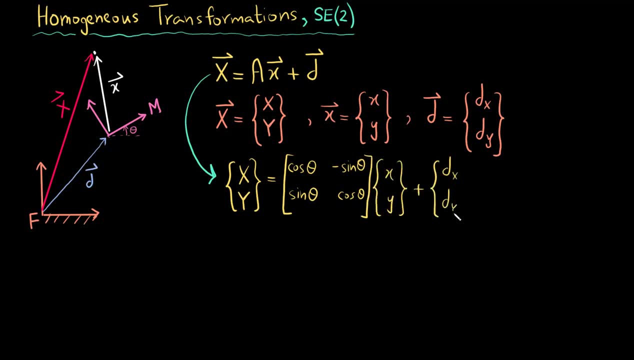 and i expand it out. i get this now. i can write the same equation in another way. we will talk about why we are writing it in this way later on, but first let me write it out as this: it is x, y and one is your first vector. then there is a three by three matrix here, with two zeros in the bottom. 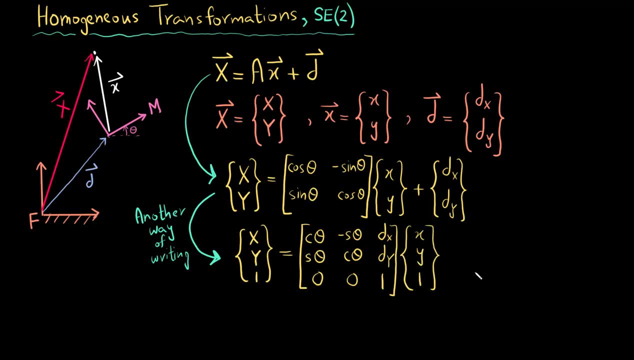 row and a one, and the rightmost vector is x, y and one. this three by three matrix is called the homogeneous transformation matrix, and i can write the same equation in a more concise form in this manner: the big x and the small x are not just the x and y coordinates of a point, but they are. 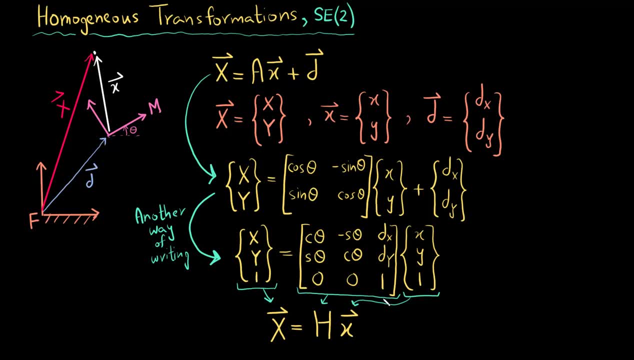 a three cross one vector, with the first two elements being the x and y coordinates and the last element being a one. if i have a look at the homogeneous transformation matrix, i notice that there is a rotation matrix tucked away in one corner and there is a displacement vector tucked. 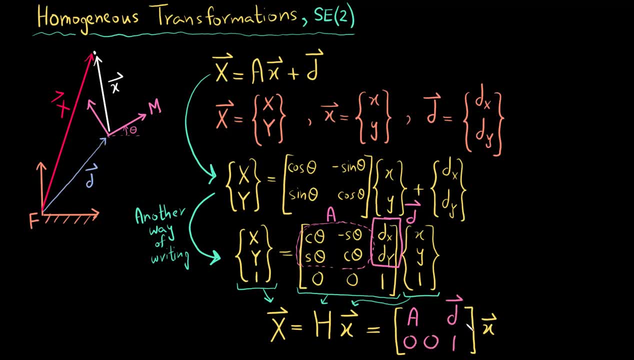 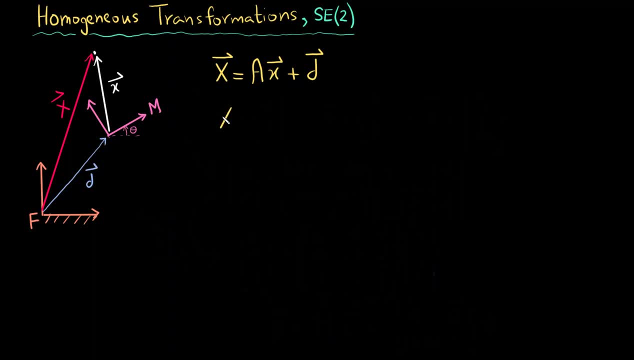 away in another corner so i can write homogeneous transformation matrix in this manner. all of this is always good to know, but the takeaway of this is that you can write this equation in this manner: so big x equals h times small x, where the homogeneous transformation matrix can. 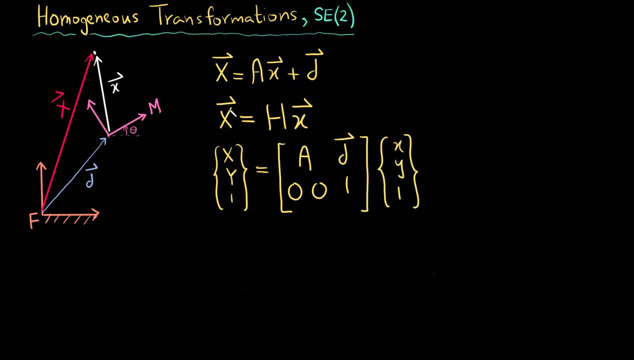 be written in this manner, which is a combination of the rotation matrix and the displacement vector. this equation that i have put a box around is the one that you should remember. the h is the homogeneous transformation matrix, or it is also simply called a transformation matrix. here is how you should. 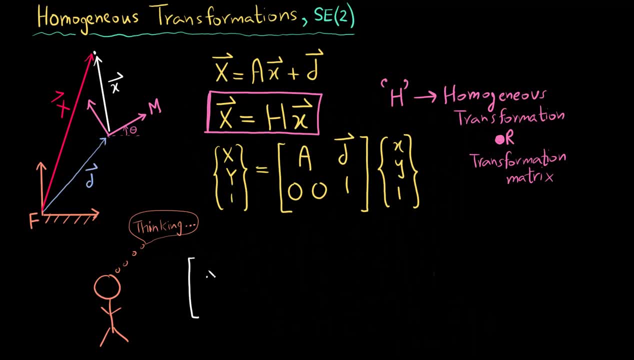 start thinking about this homogeneous transformation matrix, you notice that there is a rotation matrix within it and there is a displacement vector. so this homogeneous transformation matrix is a matrix that takes the fixed frame and it displaces it by the vector d and then, once it is displaced to its new location, it rotates it about an angle, theta, in the counterclockwise direction. 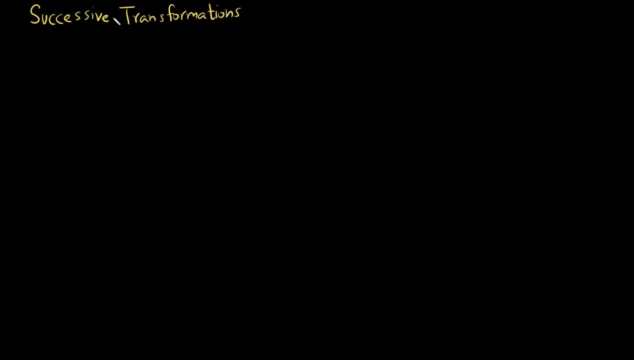 now let us see how we can use homogeneous transformation matrices for successive transformations. so here is a fixed frame drawn and there is a displacement by a vector d1, which takes the fixed frame to the first moving frame, m1, which is rotated by an angle of theta1, and then there is a displacement d2. 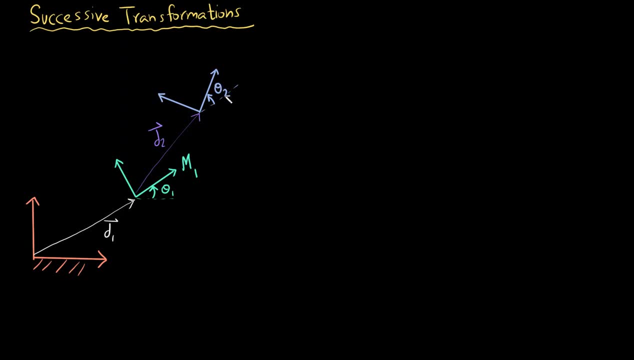 which displaces the m1 to another location and then rotates it by theta2, and i call this final frame as my moving frame. 2- m2. here is the point expressed in m2 and here is the point expressed in the fixed frame. now, if i just write it out more explicitly, the a1 would be a rotation matrix of theta 1. 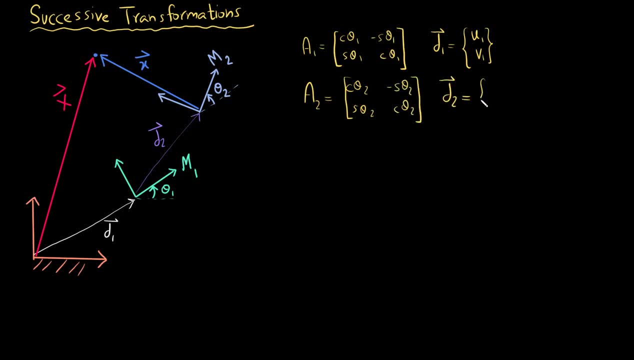 the a2 is going to be rotation matrix of theta 2, and d1 and d2 are just u1, v1, u2, v2. now, in the previous videos we have derived this equation right here, which is big x. x equals a1, a2, x plus a1, d2 plus d1, where the last two terms show the displacement and the. 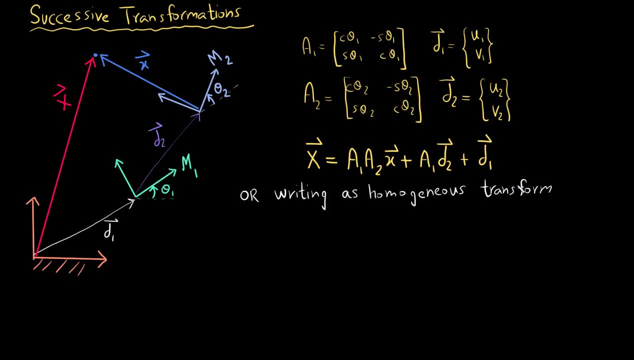 a1- a2 term shows the rotation. if i were to write the same equation out in the homogeneous transform, so i can say that the first homogeneous transform, which is h1, takes the fixed frame and moves it to the m1 frame, and the second homogeneous transform takes the m1 frame and moves it to the h2 frame. 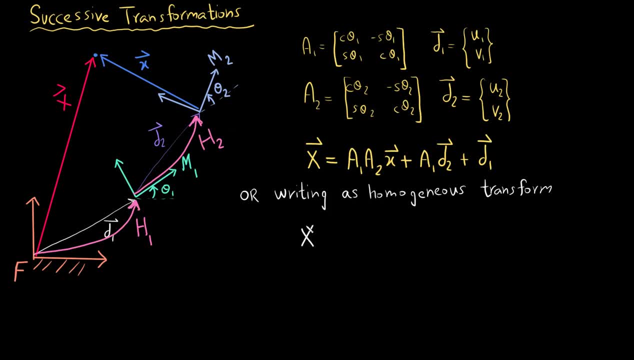 so i can just simply write all of this equation in a very concise form, which is: big x equals h1, h2, x, and, of course, notice that this is just another way of writing this equation right here. if i want, i can write it in a more expanded form in this manner and if i